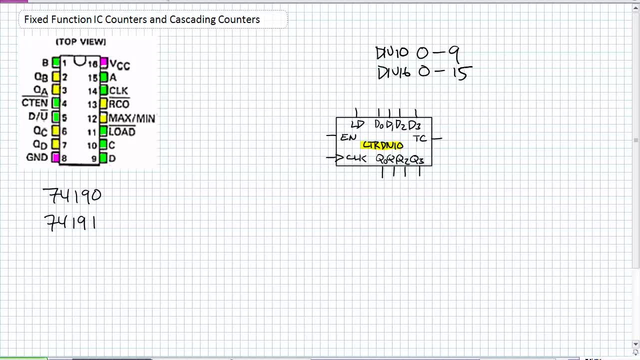 The outputs. What are the outputs? The critical thing, what are we looking for? It's the outputs right here. Those are the ones that go from 0 to 9.. Q3, it's the MSB. Q0, it's the LSB. 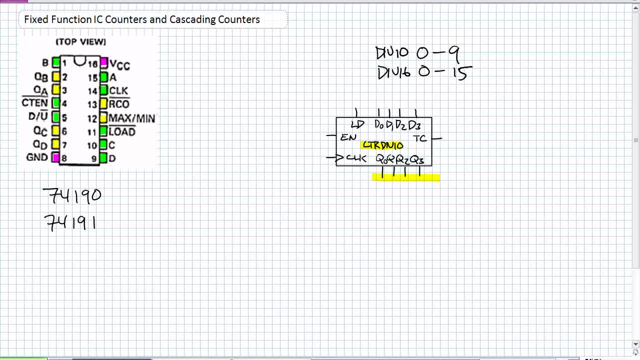 There are other outputs which we'll go over in a little bit here, The inputs. So here's an input, It's a clock signal. Obviously it drives the synchronous counter. Okay, all stages for that synchronous counter, get that same clock. 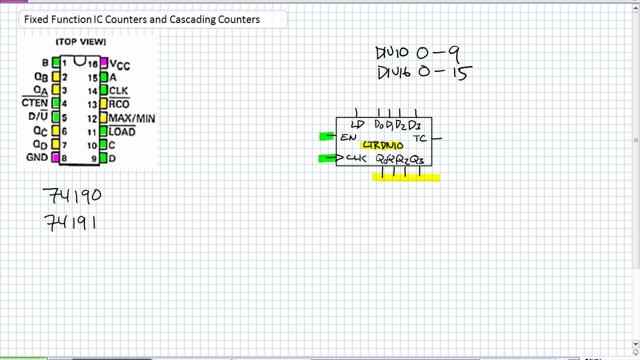 What is this enable signal here? Well, it's an enable, Okay, it is allowing that clock to count when it's enabled. What are these other things at the top here? Okay, those are data inputs and the load input, Those data inputs. 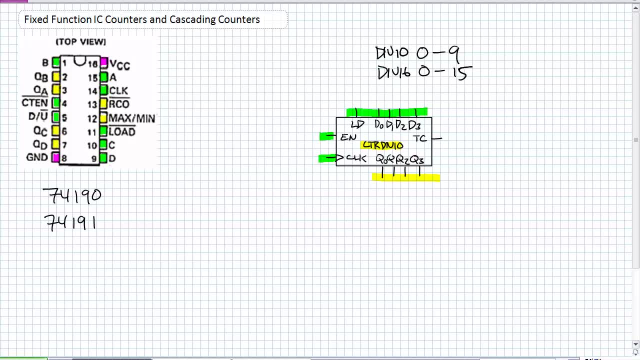 D3, the MSB down to D0.. It's kind of like a preset. And what is the load? Well, that is what you're presetting it to. They're kind of like a combination of presets and clears, And again, this is just a vanilla description. 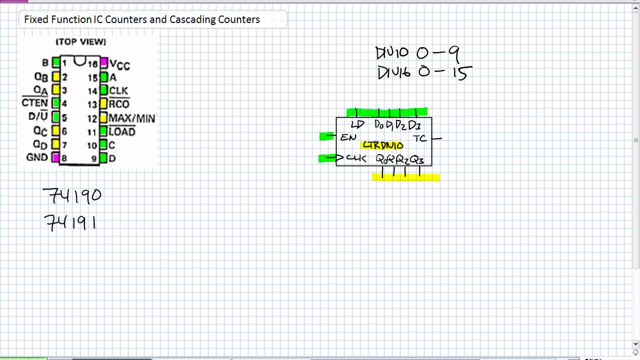 of this whole thing here. When the load command is issued- ie load something- what that counter does, it takes that D3 to D0. And input and sets those outputs to equal D3 to D0.. Okay, so I can, perhaps you know, start at 6, count up to 9.. 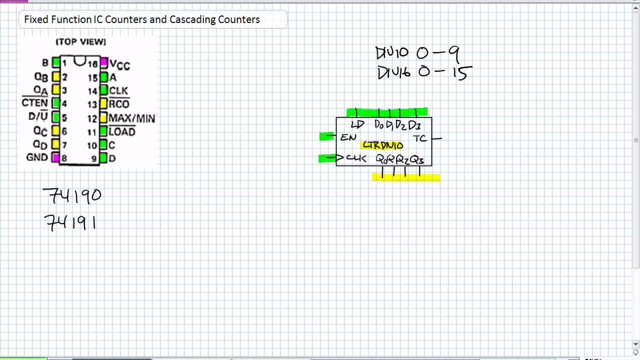 And then if I want to load that 6 again, I'd start up at 6 and go to 9.. Okay, and additionally, I mean, if I start at 6 and go to 9, if I'm not loading 6, where would I go to? 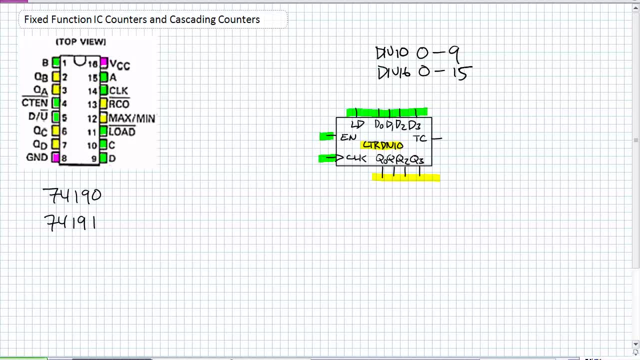 I'd go to 0. So you could potentially use those as inputs. This other thing TC to the right-hand side. that's what's known as terminal count. It is also an output. What terminal count in its most general terms? 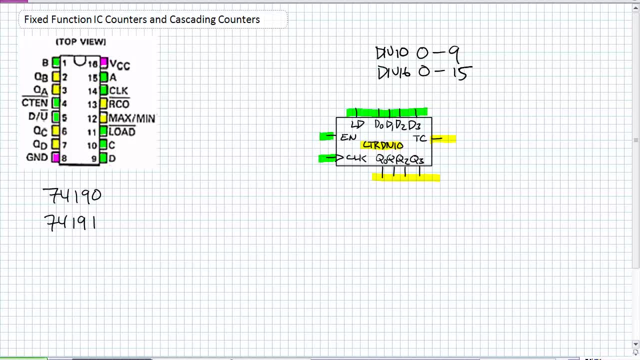 is. it's a signification: Okay, I have reached my maximum. or, in the case of a down counter, my minimum count sequence. So what that terminal count is saying: okay, this modulus 10 counter has reached its maximum. Let's assume it's an up counter. 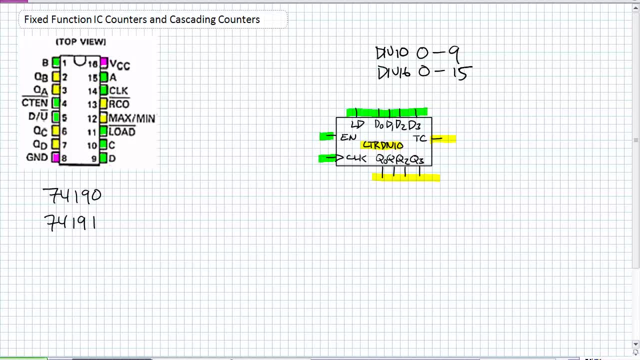 And basically it's signifying: hey, I'm at position 9.. And what's neat about that terminal count? and, by the way, it is called other things: a max min position or a ripple count out. there are a number of different names. 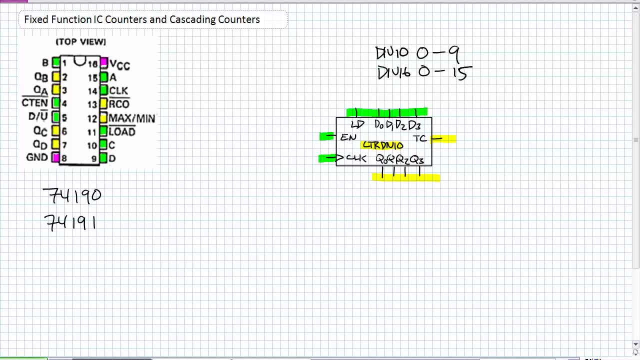 but the general terminology for it is called terminal count. Okay, it's reached its maximum or minimum in that sequence, but that can be used to enable other devices downstream. Okay, let's go ahead and see what I'm talking about here. So consider this arrangement here. 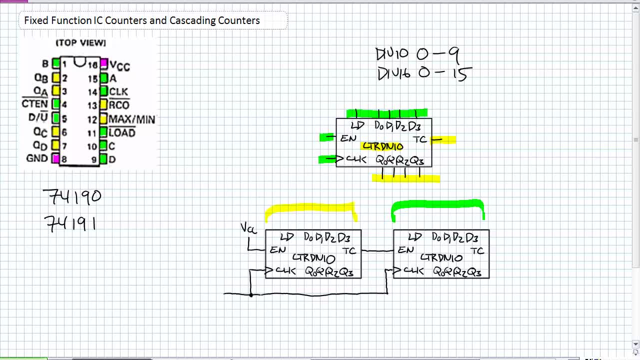 where I've got a low order counter and I've got a high order counter. Both of them are modulus 10, meaning the low order will count from 0 to 9, and the high order will count from 0 to 9.. 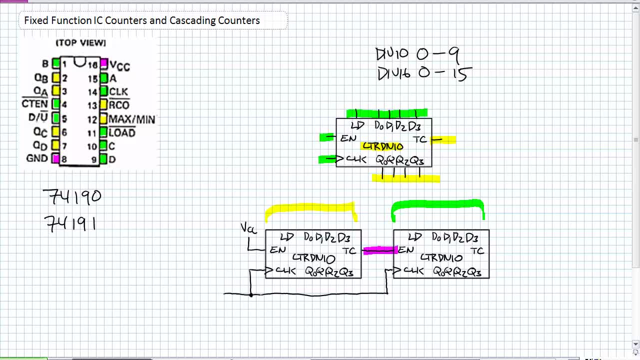 What's the advantage of something like this? Well, it's this relationship right here between terminal count and the high order count. Consider all counters. stages are currently at 0,. okay, It's zeroed out. Notice the clock. It is tied to every single one of them. 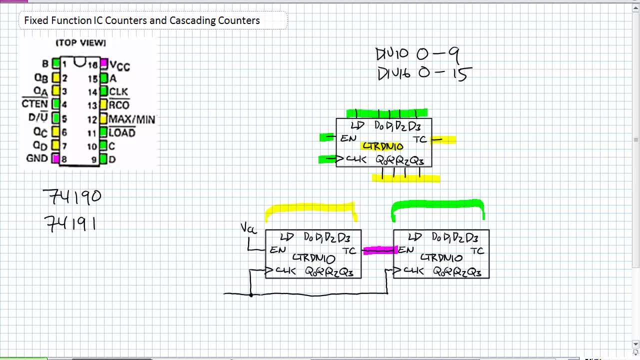 What is the terminal count for the low order counter? Well, it's not reached its maximum so it's probably low and it's going to count up on that first clock signal. Notice this high order. It's also getting the same clock signal. 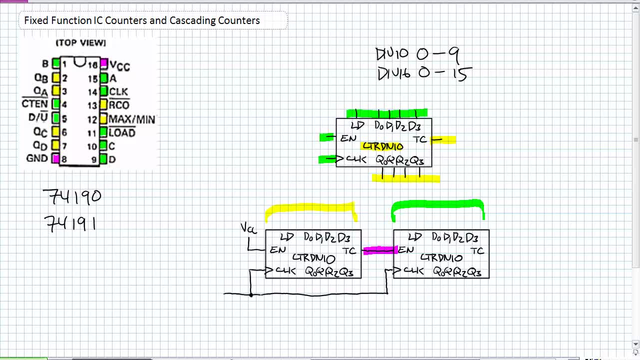 Is it enabled? The answer is no. it is not enabled because the terminal count for the low order is still low. Okay, What happens? The next clock signal counts to 2, 3,, 4,, 5,, 6,, 7,, 8, 9.. 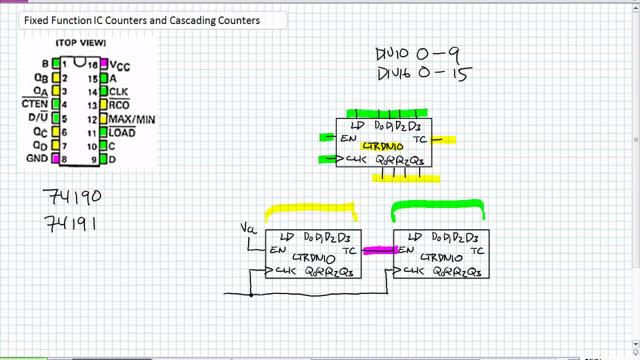 It has reached its maximum, the low order, at which point the high order is finally enabled, and the next clock signal. what happens? Well, what happens is the low order recycles to 0, and the high order is incremented up to 1.. 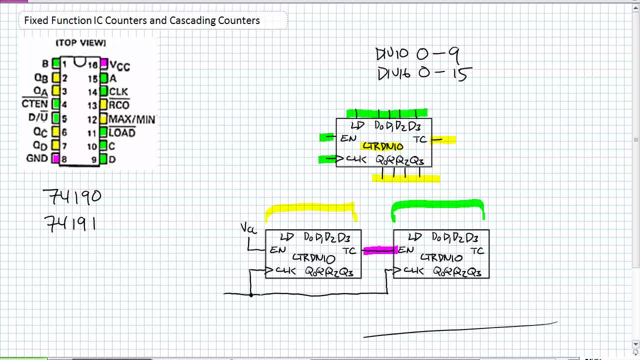 If you can imagine what's going on here- and I know this is, we're going to have to read from right to left: It's going 0, 0, and then it goes to 0, 1, all the way up to 2,. 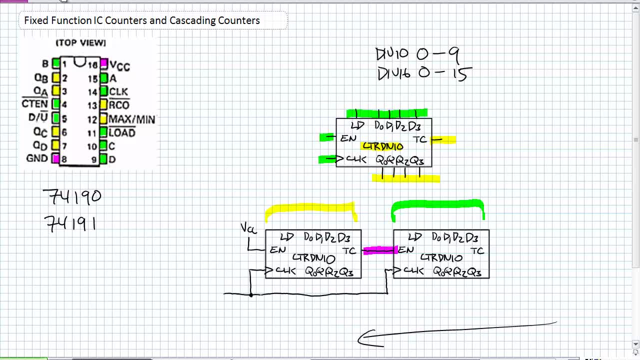 to 0, 2, all the way up to 0, 9.. The next clock pulse comes along. What have we incremented up to 1, 0, 10.. Okay, If again we're reading it backwards. 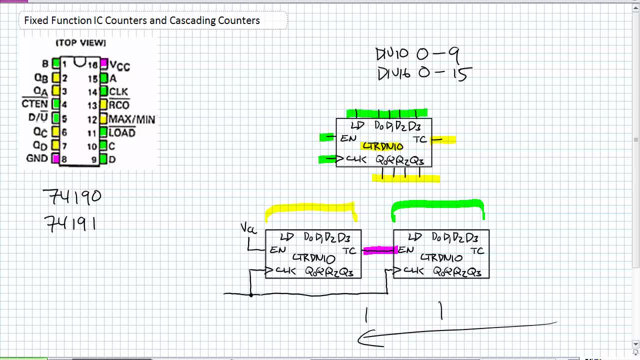 right to left there. Next clock sequence: what happens? 11,, 12,, 13,, 14,, 15,, 16,, 17,, 18, 19.. The terminal count goes high. The next high order counter is enabled. 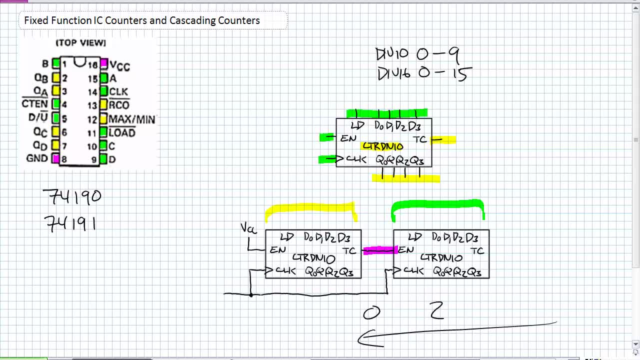 Next clock, pulse 20.. What are we creating here? We're creating a, basically a cascaded arrangement between two modulus 10 counters, Which enables us to create- if this is a whole big box, here it's a modulus 100 counter. 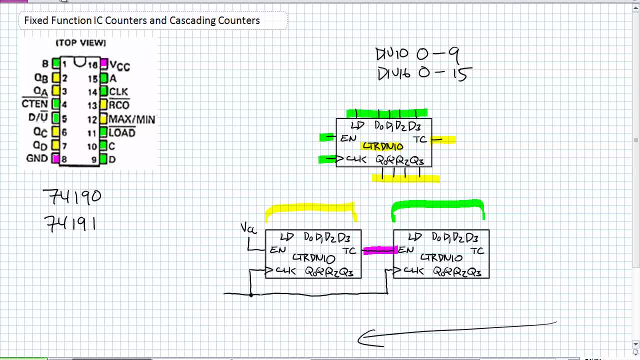 Which will count from 0, 0, up to 99.. You want to create 1,000 modulus counter, add another modulus 10 counter at this end, which is enabled by this high order. So these cascading arrangements for a fixed function integrated circuit, you can use them. 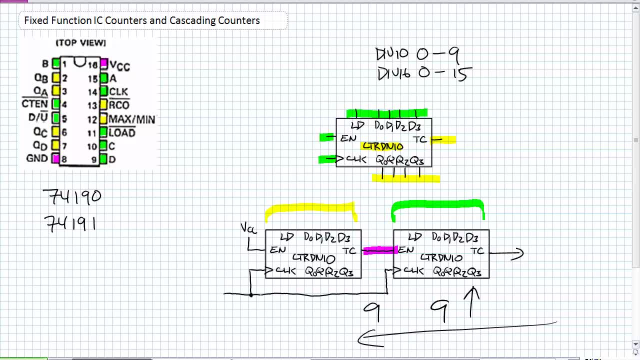 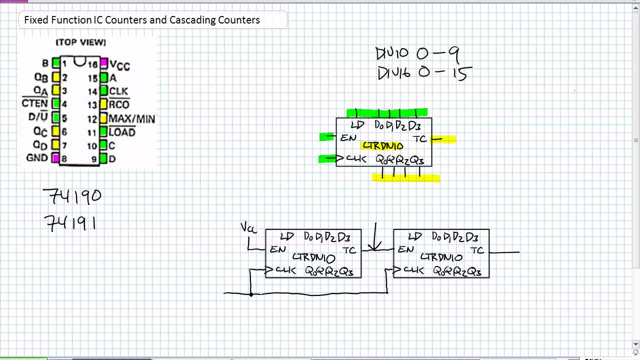 to create higher count sequences than what they are by in and of themselves capable of doing. So a quick note about the terminal count signal for a modulus 10 counter That goes high or is asserted, Pretend it, you know could be an active low signal. 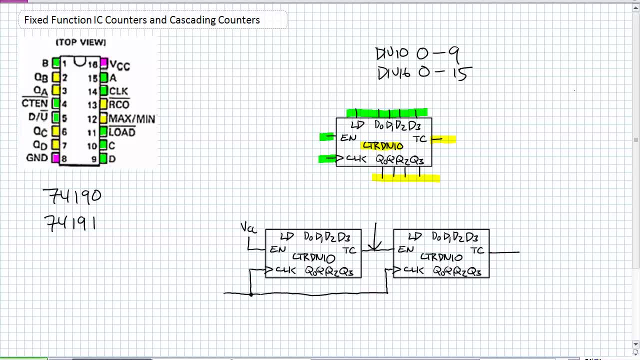 Either it could go low. Yeah, Drives me crazy too. It only is asserted a tenth of the time. So this clock frequency that's coming in. let's just do a very simple example. It's 100 hertz clock. 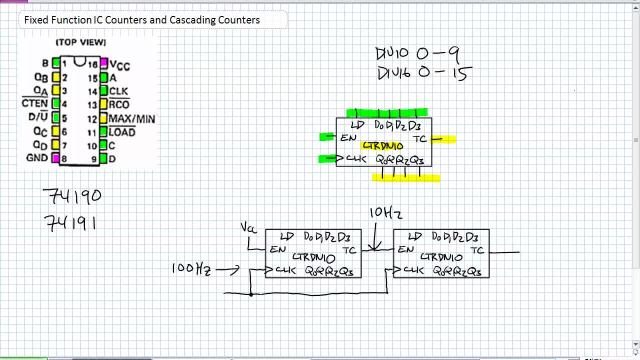 Every 10 times that is asserted. what is the frequency of this? It's 10 hertz, And then it is a tenth for this higher order one. It's a tenth of what its input enable. So what is that? 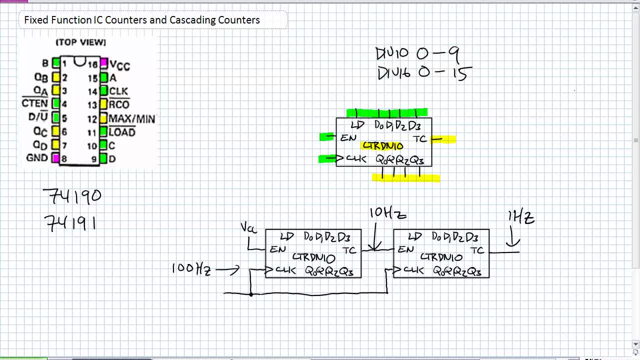 It's 1 hertz. So with modulus 10 counters we are capable of doing frequency division by 10. Whereas previously, if we were stuck with a modulus 16 counter, by using those previous stages- Q0,, Q1,, Q2, Q3, we were limited. 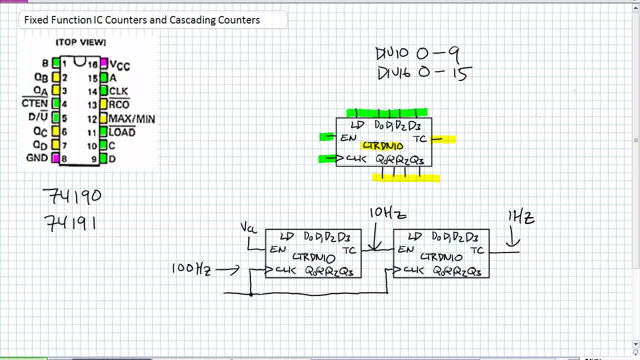 to a half a quarter: an 8,, a 16,, basically a power of 2.. We could potentially divide our clocks by 10, in this case using a modulus 10 counter. So that vanilla description right there for a counter. 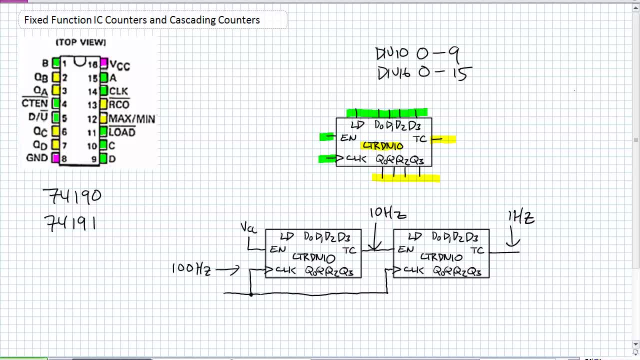 it's going to serve for a general purposes, But let's just talk about some specific counters here. Okay, Notice I did not have an up or a down input to this one. There are fixed function integrated circuits that have basically two modes: up mode and down mode. 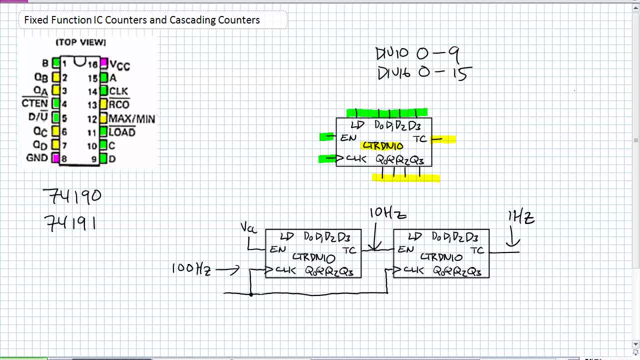 If it's a modulus 10 counter in up mode, it counts from 0 to 9 and recycles. If it's a modulus 10 counter that's in down mode, it counts from 9 to 0. And recycles. okay, as you would expect, 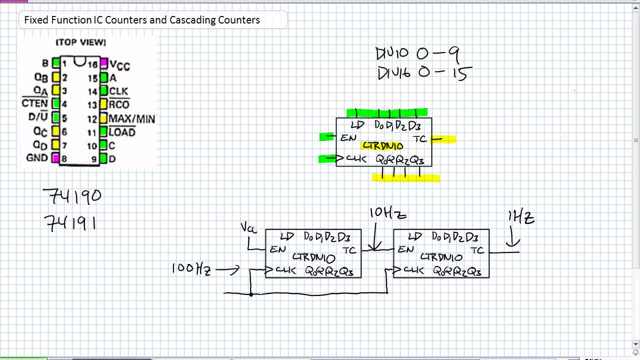 The two fixed function integrated circuits very commonly used is the 74190 and the 74191.. Okay, The 74190, it's a decade counter, ie a modulus 10, it counts from 0 to 9 or 9 to 0,, as we'll see. 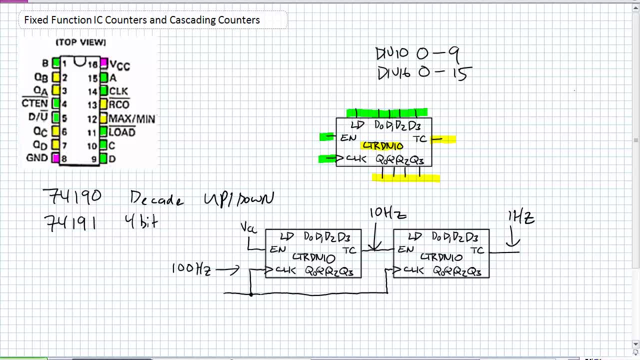 It's an up-down counter 74191, it's a 4-bit binary, full sequence up-down. What's awesome about these things? they have the same pinouts. Okay, Now let's go ahead and look at our pinout diagram. 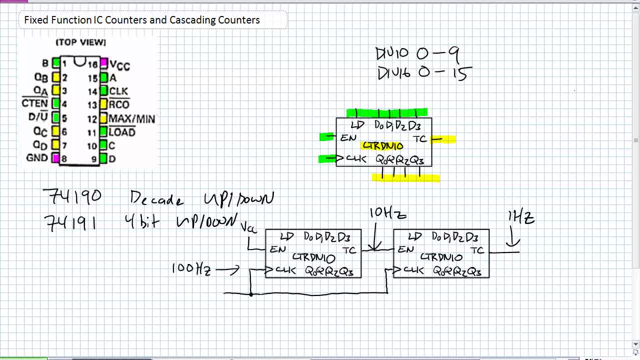 And all the things in green, those are our inputs. All the things that are in yellow, those are our outputs. All the things that are in pink are things that are make this thing work, And without them they're not going to work. 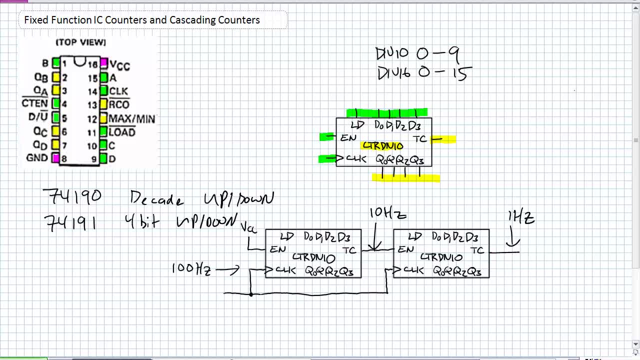 Pin 8 and 16, obviously are VCC and ground connections. Let's go ahead and look at our outputs: Pin 7,, 6,, 2, and 3, those are our count outputs from MSB to LSB. 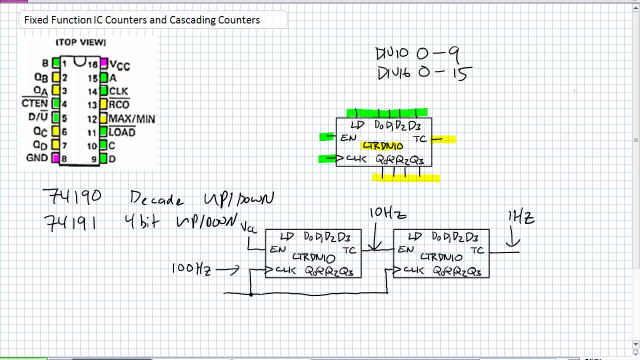 QD, QC, QB, QA. What's pin 12 and 13?? That's kind of. it kind of is two Terminal count outputs The max min. it goes high when it is at its maximum in an up sequence. 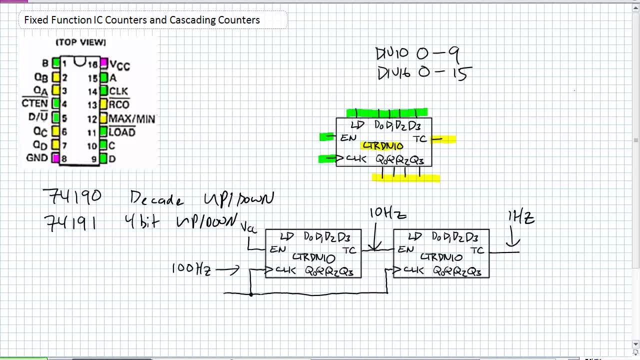 It goes high when it is at its minimum in a down sequence. So if it's counting from 0 to 9, obviously it's an up mode. It's again for 74191, I'm talking about here. 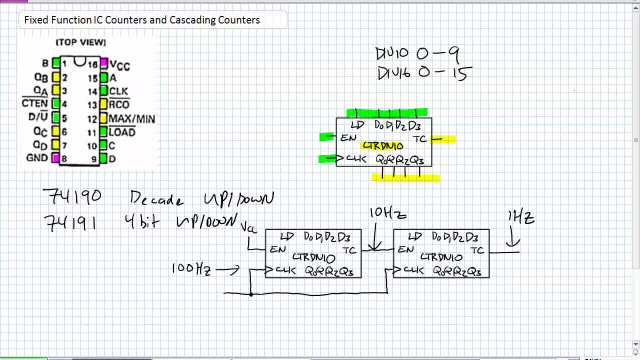 When it reaches 9, that goes high. What's number 13?? Well, that's what's ripple count out. Okay, It's notice the bar over the top of it. That goes low once it's gotten to its maximum position. 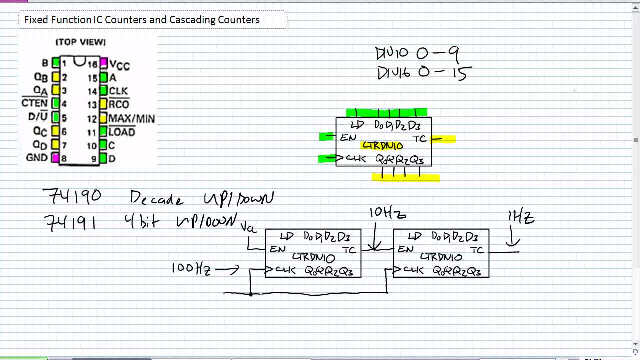 or minimum position. I don't know which mode it's in, but it's only asserted for a brief moment, So I'll show you in the timing diagrams within the data sheet what I mean by that. Okay, What are our inputs there? 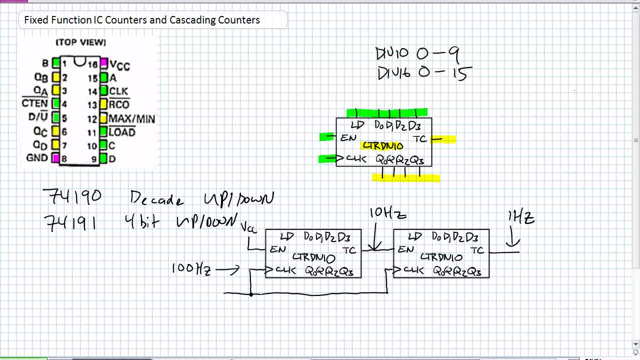 Those are all the greens. Where's our enable? Well, it's pin 4, count enable. with a bar over it, It's active low enable. So I have to have a 0 on pin 4 to even get this thing. 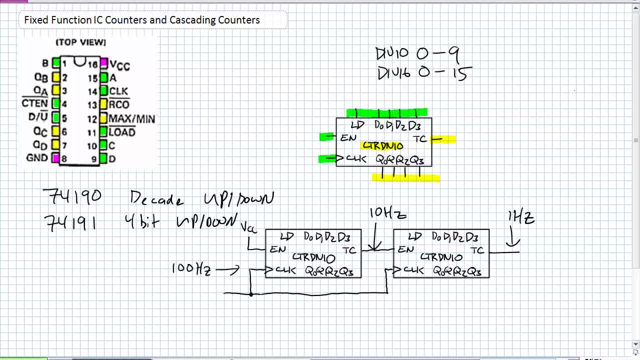 to work at all. Pin 5,. what is it? It's a single pin with two inputs on it. Okay, What does that mean? Well, if it's a single pin, it's binary 0 or 1.. When it's a 0, what mode is it in? 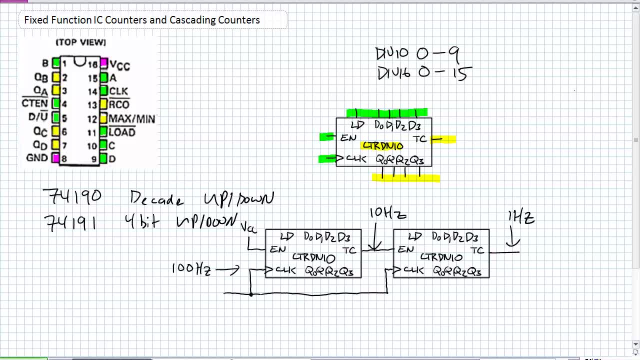 It's in up mode because notice the bar over the up When it's a 1,. what mode is it in? It's in down mode because there's no bar over it. You've got two choices, mutually exclusive, and you can neither go up and down simultaneously. 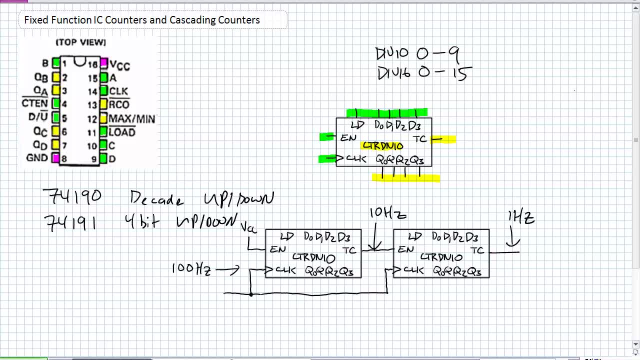 You can only go down or you can only go up. What are the other inputs? Obviously our clock, pin 14.. What are the data inputs? You know, in our general diagram over here, D3 down to D0,. 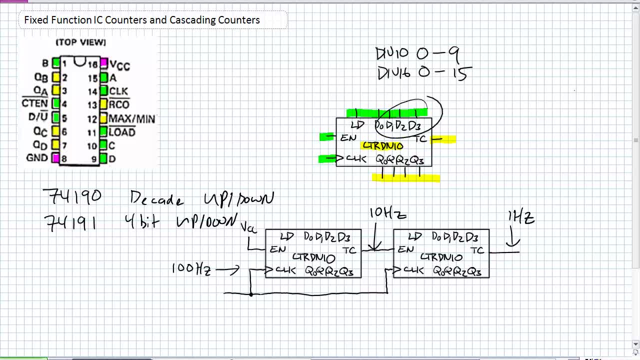 our specific diagram. this is a. somebody has made this thing and it's got its own pin outs and pin ins. Well, where's 9?? Pin number 9 is our D3.. It's called D Pin 10, that's C. Pin 1 is B. Pin 15 is A. 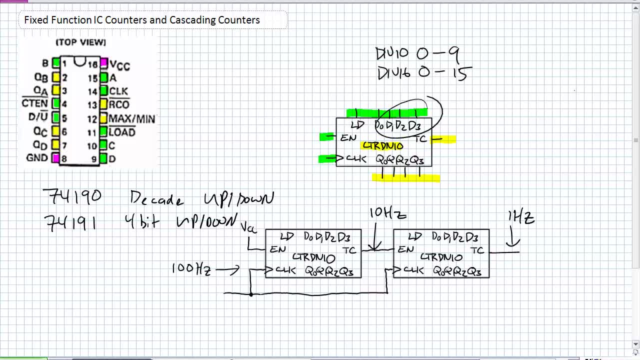 That's corresponding to our data inputs. Okay, How do I preload those? Well, with pin 11.. Okay, If pin 11 goes low, I load D, C, B and A onto QD, QC, QB and QA respectively. 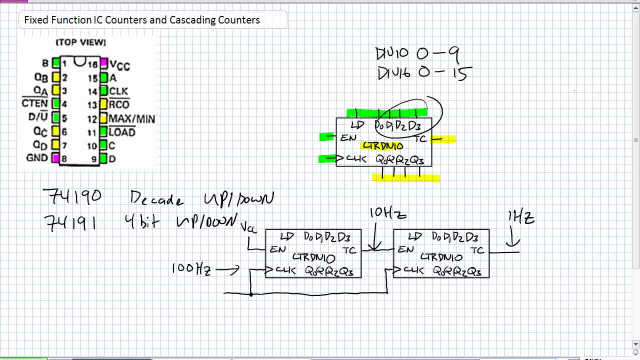 Well, I've talked about some of the basic terminology of this basic configuration, basic counter. I talked about some specific counters there And the only difference when again between the 74190 and 74191 is you go ahead and put the 74190 in up mode. 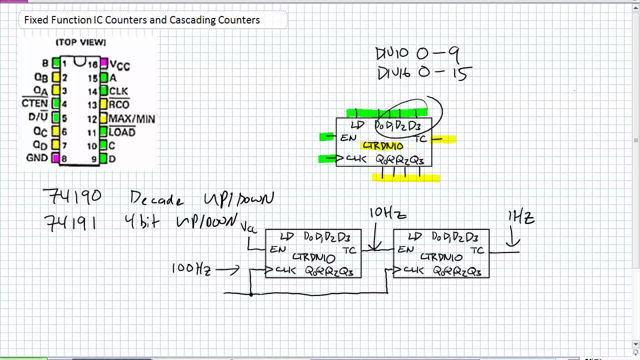 and let it count. it goes from 0 to 9.. Put the 74191 in up mode and it counts from 0 to 15.. Let's look at the data sheet specifically. I'm just going to show you some pretty neat things. 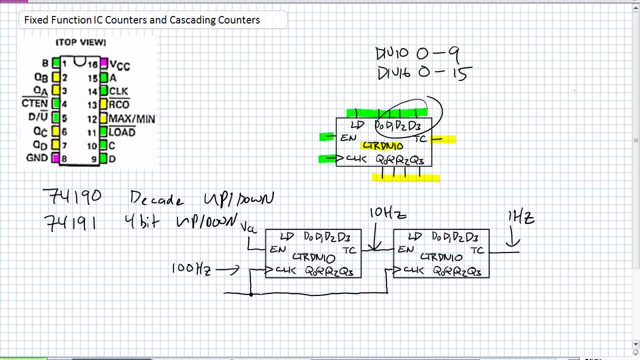 about a data sheet, the full data sheet. If you look at these things, the data sheets tell you how these things work, And this is one of those things I just can't do. all the TTL data sheets for you. Just grab it. 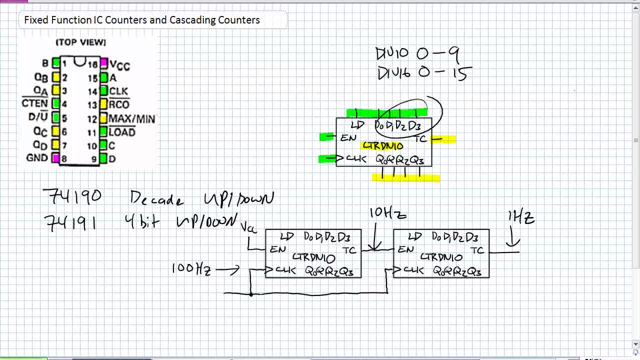 Just grab the TTL book, grab a data sheet and just look at it and start looking at how these things work. It's really neat. 74190 and 191 on the data sheet. they actually have example waveforms to see how these work. 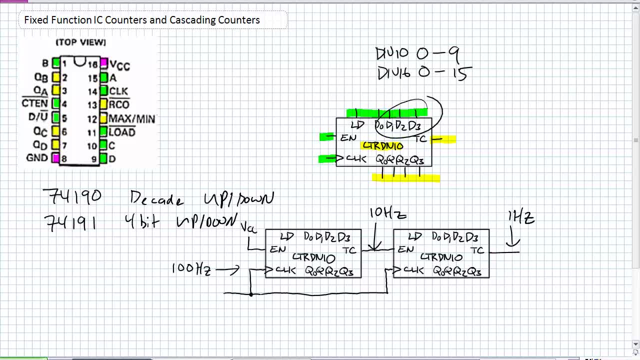 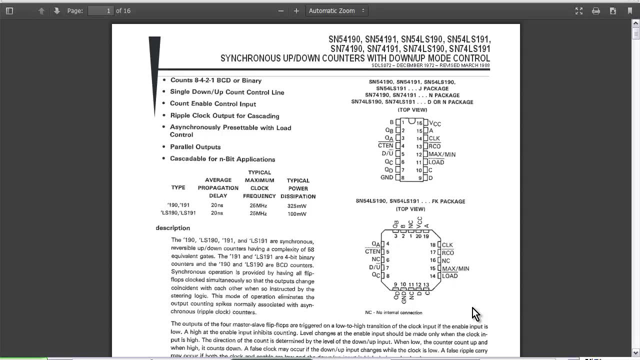 So let's go ahead and take a look at a data sheet and we'll describe exactly what I did here. Here is the 74190 and the 74191 data sheet and it's showing us our pinout configuration. And again, what is it showing us right here? 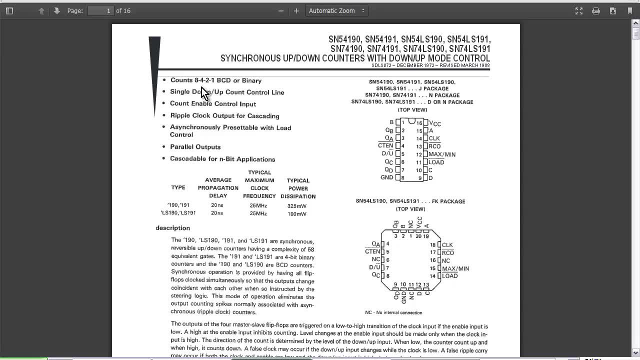 Its main function. It's going to count 8421. BCD, That's the 74190, or binary, That's the 74191.. It's got an up or down mode. It's got a count enable ie to turn the whole thing off. 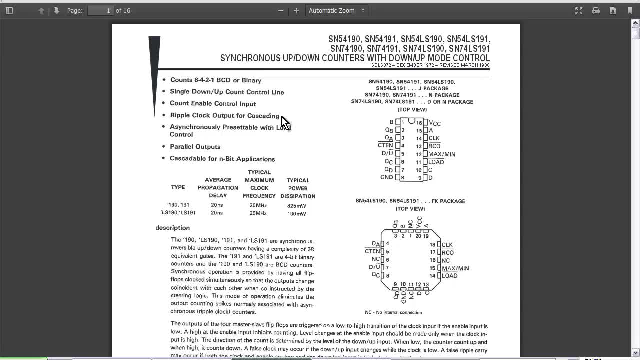 or turn the whole thing on. It's going to have a ripple output for cascading, just like we talked about there. There's basically a terminal count output in the form of the RCO and the max min that could potentially enable another device. 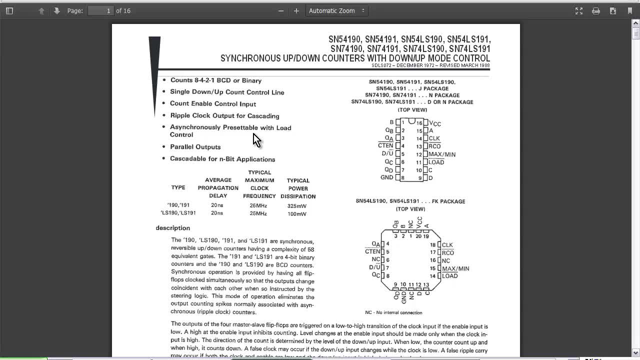 And additionally it's talking about asynchronously pre-setable with load control. That's, when load goes low, Those D inputs are brought to the Q output. and again, what are those outputs? Well, they're parallel. You know, you don't have to wait for a serial stream. 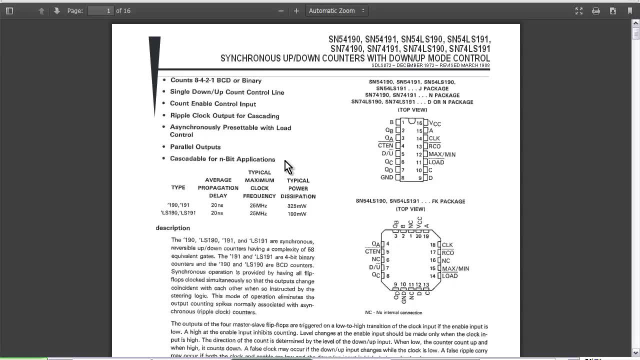 of data to come out. They're all simultaneously available and then cascadable again for n bit applications. When that letter n is in there, it's for how many n's you want, how many? what's your larger modulus? 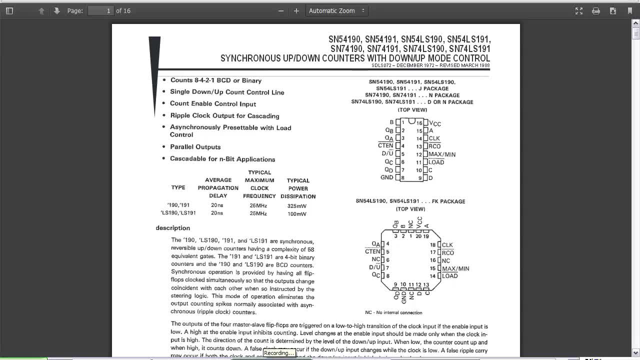 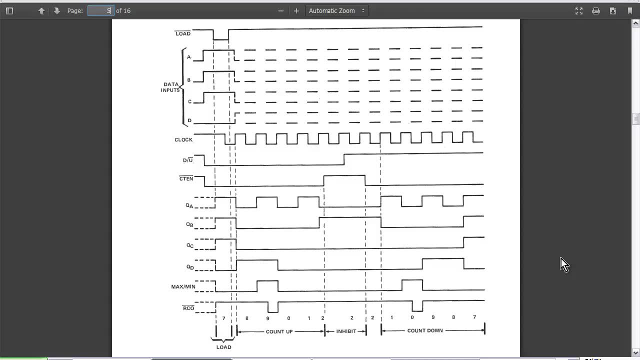 So let's go ahead and skip over to page 4 for this guy. excuse me, page 5.. So page 5 on the 74190, 74191 data sheet here. this is where the money's at here. Just by looking at it, we can see that this is where the money's at here. 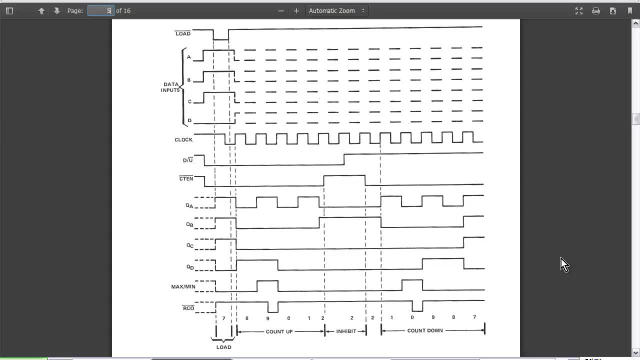 Just by looking at it, we can see that this is where the money's at here. Just by looking at it, we can see that this is where the money's at here. Just by looking at this diagram here, I can figure out how this thing works. 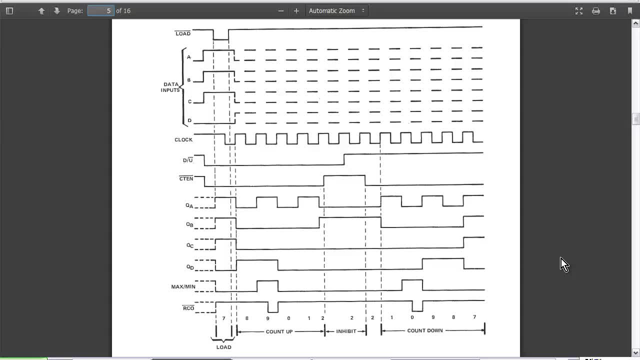 This is for the 74190, the decade counter. Notice. at this moment, here it is given an active low load. What is its loading? It's loading 0111, ie 7.. What happens? Well, obviously, our output should go to 0111, ie 7.. 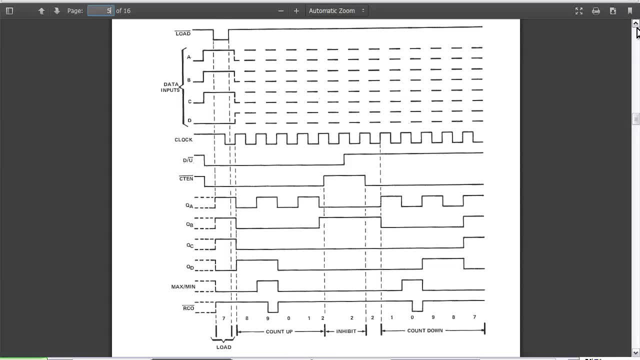 So that's what it's showing you. It's showing you an active low load. Take those data inputs, Load them onto the outputs. And what is all this stuff right here? It means it doesn't matter. because it doesn't matter what's? 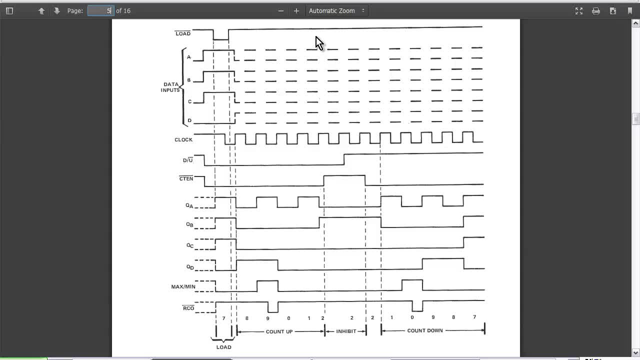 on those data inputs. It never goes low again. okay, It never loads anything again for this particular sequence. Notice here we've got a count: enable. It's enabled because it's low, It's not enabled. Look what it's telling you. 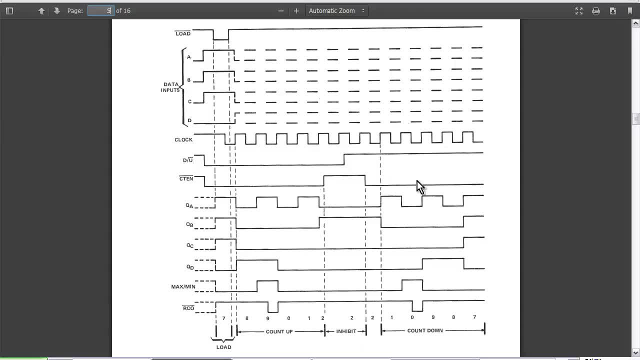 It's inhibiting count operations, okay, And at which point it goes low again, it will be enabled. Notice here too. here's our other input: down and up. It's two choices. What does it mean here? okay. 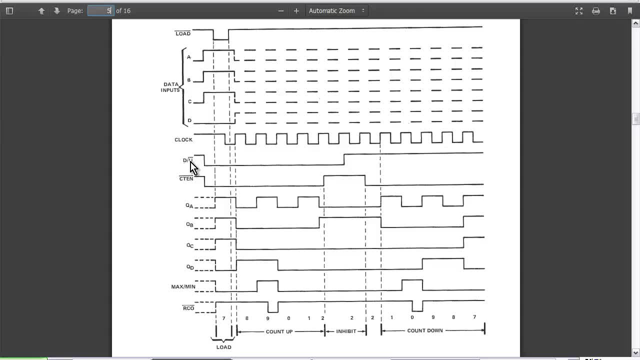 See, D has no bar over it, U has a bar over it, So it's an active low up. So between: for this section right here, as long as it's enabled, it will count up For this section here as long as it's enabled. 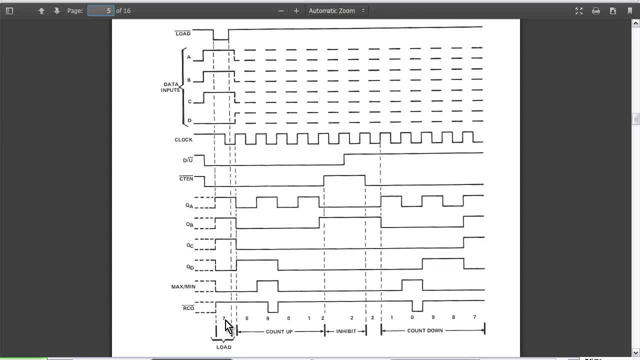 it will count down, So we started at 7.. We are enabled. What does it do? We're in up mode. We count to 8. Look at what happens to our maximum minimum there. It's telling us decimal 8.. 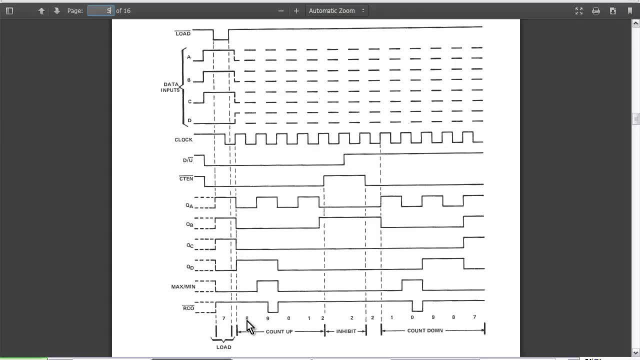 How can I read that It's 1. 0. 1. 0. 0. 0. 0.. That's what that means, right there. Now I count up again, I go to 9. 1. 0. 0. 1.. 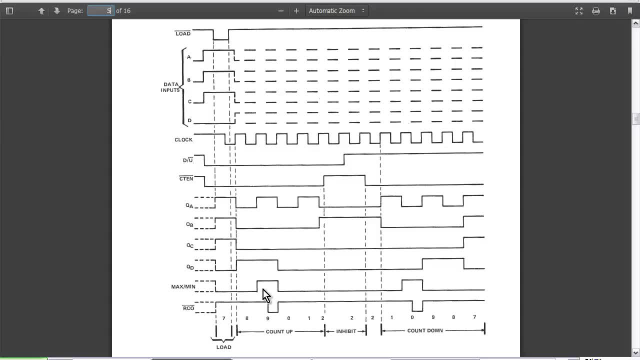 Notice what happens to maximum minimum. I'm at the maximum of my count sequence because again we're at a decade counter. Notice what happens to RCO: It goes low, but it's a brief pulse okay, Whereas maximum and minimum goes high the whole time. it's 9,. 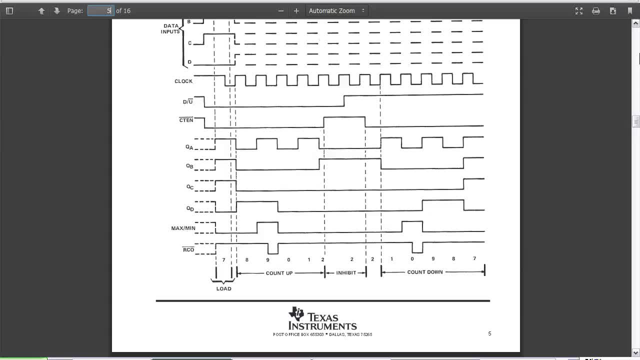 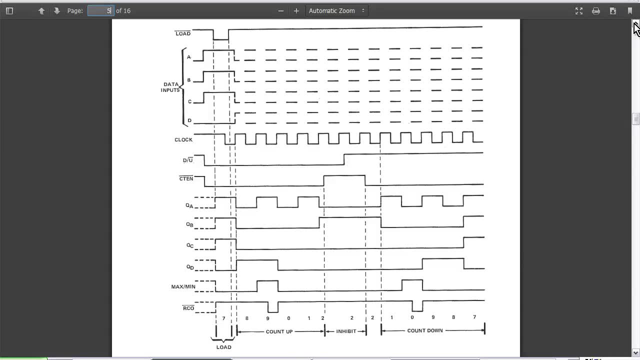 RCO goes low only for a brief moment, That could potentially, because it's active low, be used to enable it to go down. That could potentially, because it's active low, enable another active low-enabled device like another 74190.. 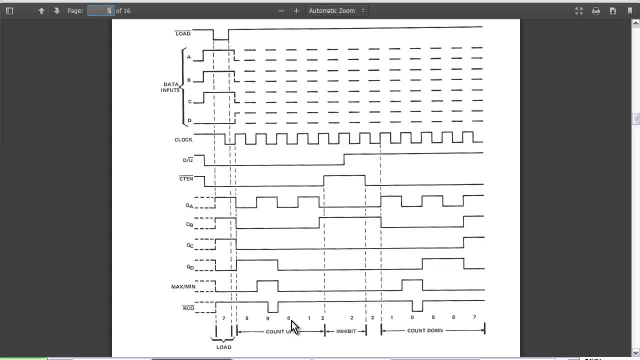 Again we are in count up mode. We go to step 0,, 1,, 2.. We are inhibited. We stay at 2.. We're at 2.. Now we're in down mode, though, The next positive edge. we were at 2.. 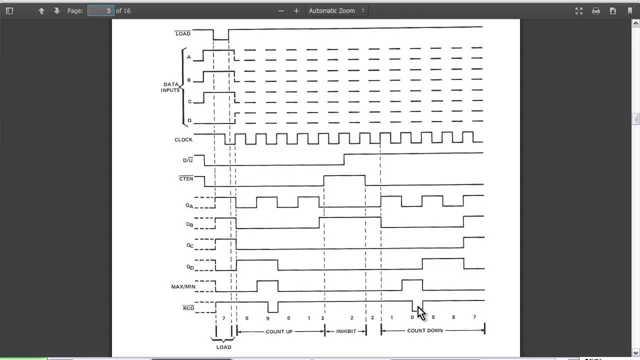 We go to 1.. Now we go to 0.. What happens to RCO? It goes low. What happens to maximum and minimum? It goes high. okay, It's, those are kind of your combined terminal count outputs. there It's telling us it's at the either the maximum or minimum. 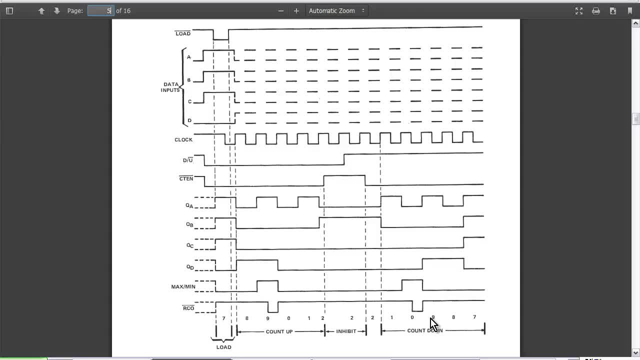 Again. next positive edge comes along. We are in down mode. We're currently at 0.. What's it do? It recycles to 9.. It goes to 8.. It goes to 7.. And again, if you want those binary inputs. 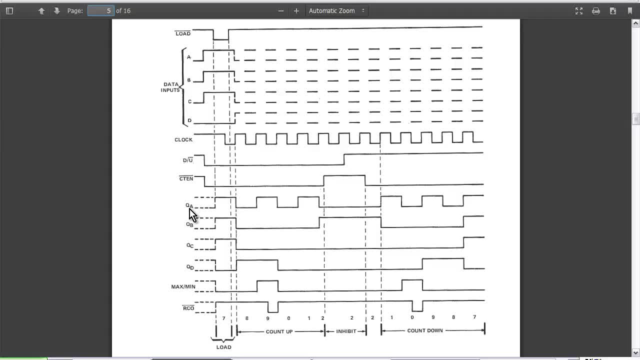 for the decimal equivalent. where are they? They're right there: QD, QC, QB and QA. So not only does the data sheet give you those pin out configurations, it's also giving you how this thing functions, in addition to all that performance data. 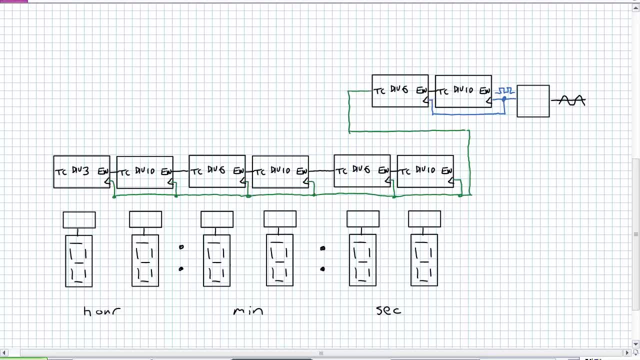 As we wrap up our lecture on fixed function integrated circuit counters and cascading counters, I would be remiss if I did not include this in the video, This example here that has appeared in pretty much every digital electronics textbook since the Roman Empire. This is the classic digital clock application. 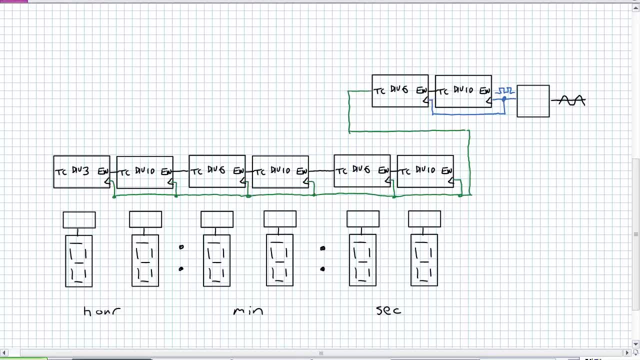 of cascading counters. What we've got in the upper right-hand corner is, assuming, 60 hertz AC. I'm not certain if the Romans had 60 hertz AC. If they had something different, they'd have to do something a little bit different here. 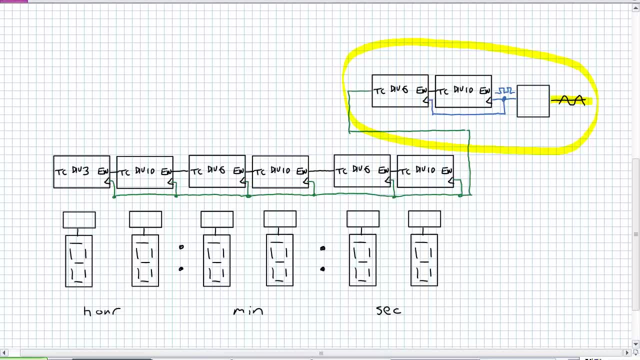 But what we're feeding it is to what's called a wave shaping circuit. You may have done this already in semiconductor devices and circuits. If not, you'll probably do it this quarter. What it's creating? it's creating the same frequency. 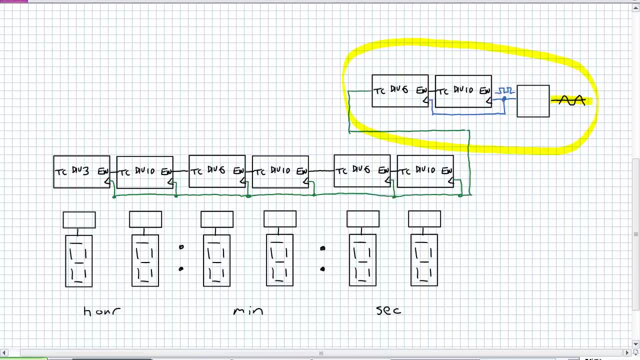 Okay, so that output still has 60 hertz output. However, it's TTL compatible. It goes from 0 to 5 or in this, if you want to do CMOS, you could 0 to 3.3. But again, this frequency is still the same. 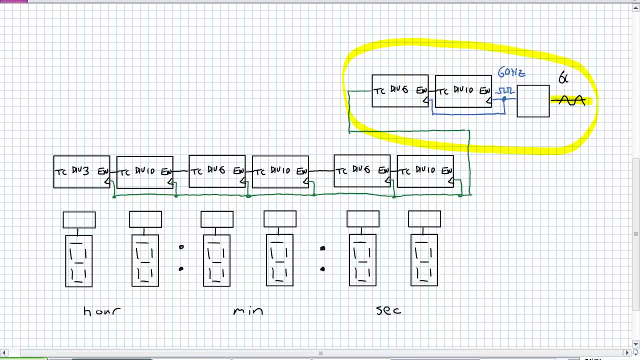 It is no longer zero centered. So we've got 60 hertz AC being fed into our wave shaper and we've got 60 hertz 0 to 5 TTL compatible coming up. What is it being fed into? It's being fed into a modulus 10 counter. 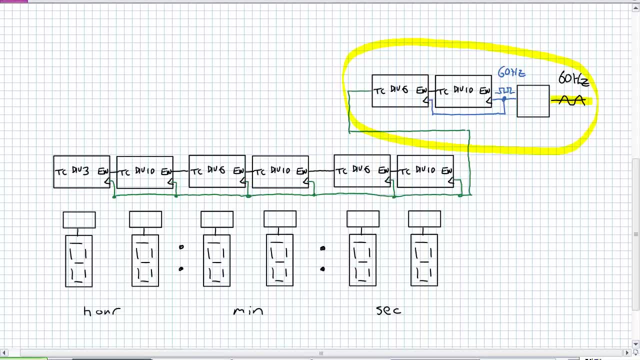 and the modulus 6 counter. What is that whole thing taken together? It's a modulus 60 counter that counts from 0, 0 to 59.. Okay, it's modulus 60.. So if you look at the terminal count right here, 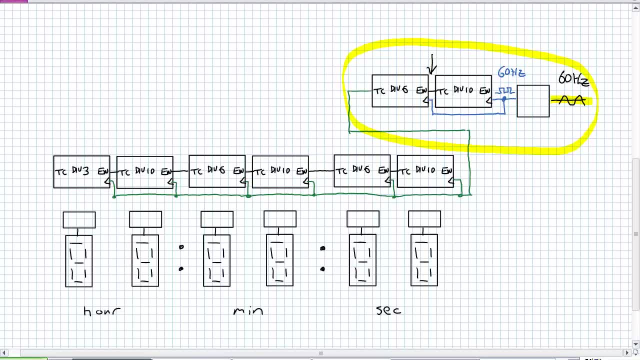 that goes high every 10 times that, one of every 10 times that the low order counter goes through its sequence. So what is its frequency? It's 6 hertz. Okay, what's the output here for the terminal count of the modulus 6 counter? 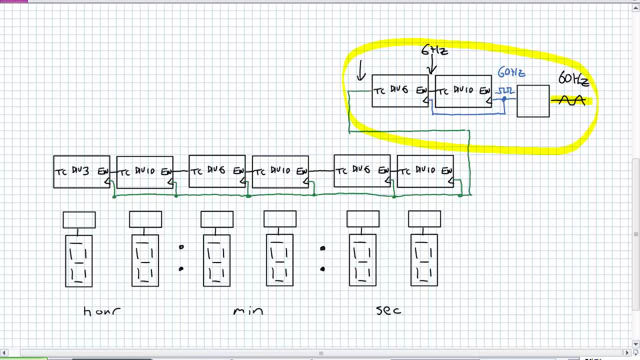 Because again, it goes from 0 to 5.. It's going high when it reaches 5, ie once of every 6 of them. So what is the frequency there? It's 1 hertz, So 1 cycle per second. that is now our new clock. 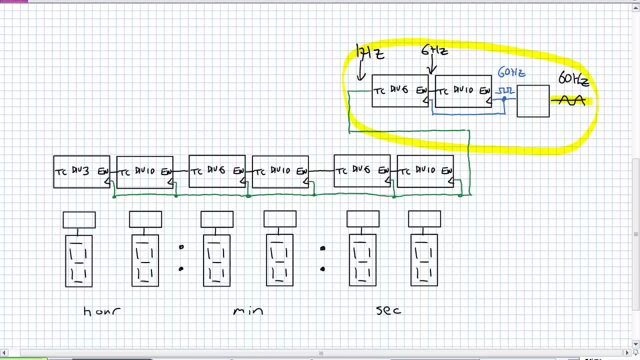 That's the green line. Look at this. That green clock, that new green clock which has been generated, has now being fed to our hour, minute and second display, And what we have shown here is again is 3 separate sections. Here I've got seconds, minutes and hours. 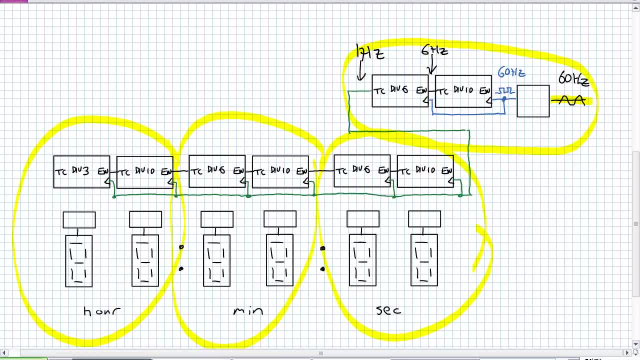 They're all being clocked simultaneously. What is the seconds? It's a modulus 60 counter consisting of a 10 and a 6.. When that low order is enabled, the terminal count goes high every 10th of a time. So it counts from 0 to 9, at which time the higher order second. 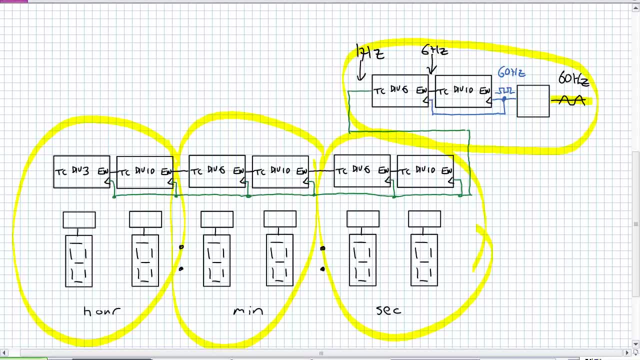 is enabled and it goes to 10,, 11,, 12,, all the way up to 20,, 30,, 40,, 50,, 59. And then it enables this one And that first minute is incremented And same thing. 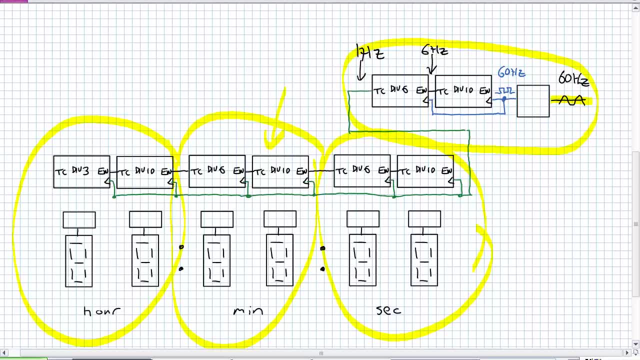 It's a modulus 60 counter And it goes from 0 to 59, at which point the hour is enabled, And what we've got here is a 24-hour clock example. The only way time should be presented is in 24 hours. 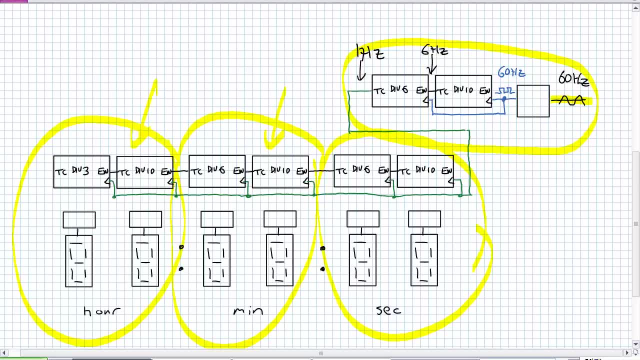 What this thing is going to do is going to count up to 24.. And then I have not drawn a reset on this here, but it was going to have to go back to 0, 0, 0, 0, 0.. 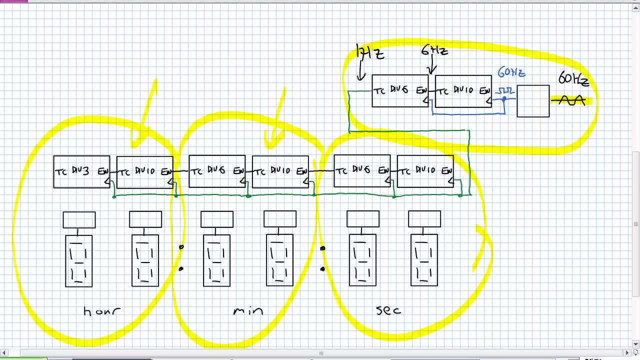 What is being presented below here? Well, that is our display drivers and our displays for each individual digit within the hour, minute and second, And what that's implying is, there is the outputs for that stage. go to that one, into that driver. 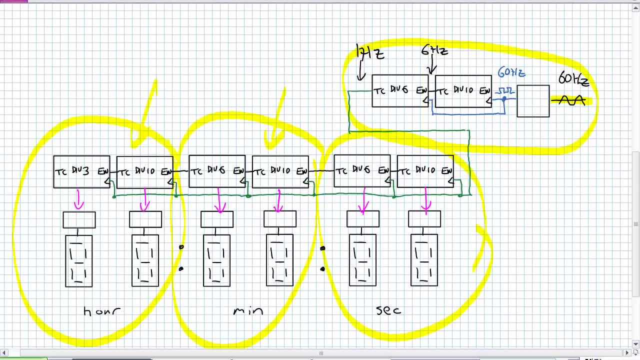 which goes into a seven-second display, And if we wanted it to be especially cunning, we could potentially do a single driver and display multiplex at an extremely fast rate for all six of those displays. It's an application of a cascaded counter. 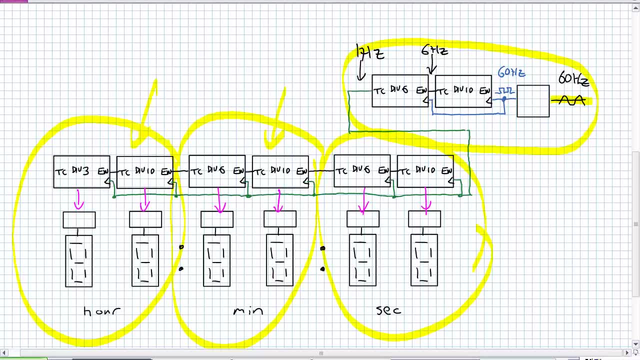 Basically the high order. a second only enables the low order minute every 60th, every 60 times, Once every 60 times, as you would expect. So it's got to count from 0 to 59 to get a full minute. 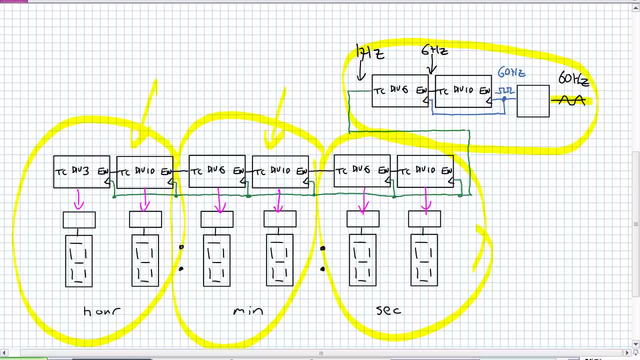 Then you go up to 1 minute, Then you've got to have 60 minutes to enable the hour. Classic example of cascading counters: here Again, just think of it in a vanilla terminology If you want to do a specific device like a 74190 or 191,. 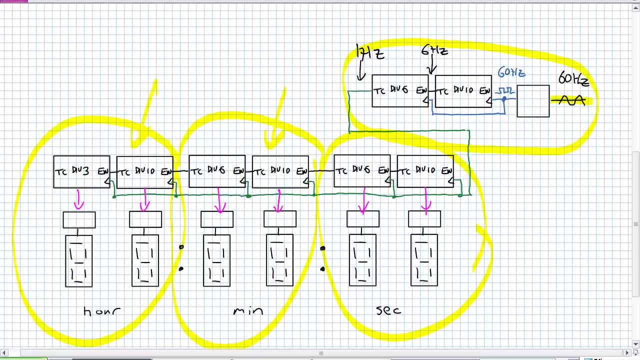 you might have to use the data sheet because, as I showed, if those were active low enables you'd have to have a minimum terminal counts. This concludes this portion of the lecture. Let's move on to the next topic.